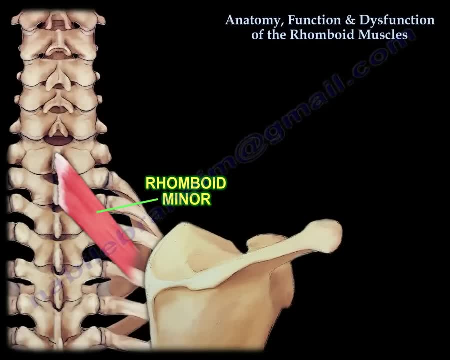 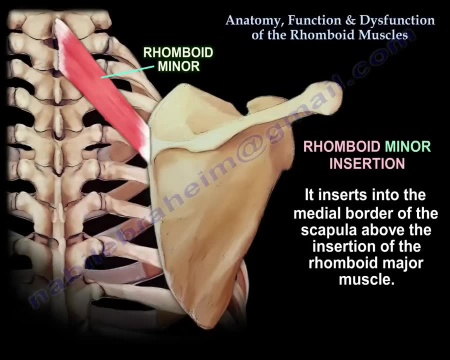 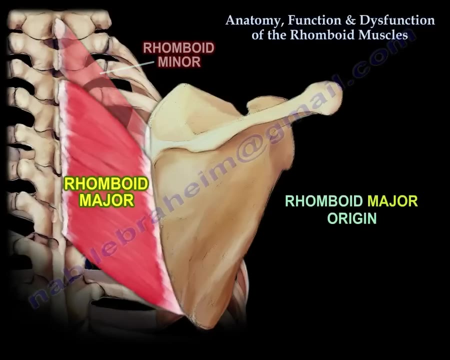 It inserts into the medial border of the scapula above the insertion of the rhomboid major muscle. The Rhomboid Major, It truees from the spinous processes of T2,, T3,, T4, and T5 vertabrae. 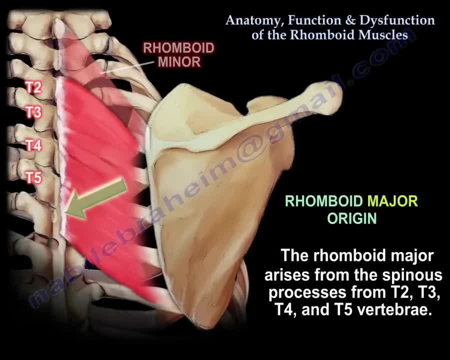 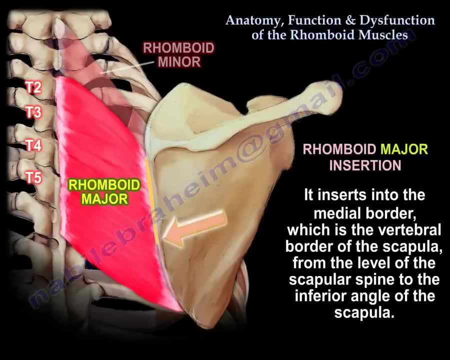 The rhomboid minor is the dariusus vellansus or rhombus Insertion. It inserts into the medial border, which is the vertebral border of the scapula, from the level of the scapular spine to the inferior. 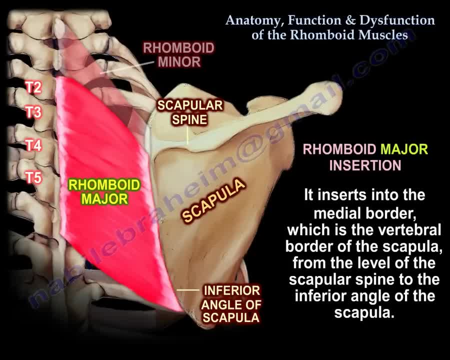 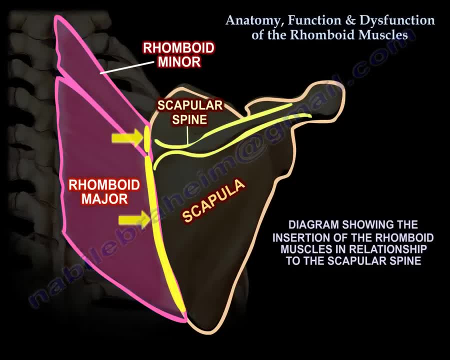 angle of the scapula. Here is a diagram that shows the insertion of the rhomboid minor and major in relationship to the spine of the scapula. Here is a line parallel to the spine of the scapula and here is the line of the separation. 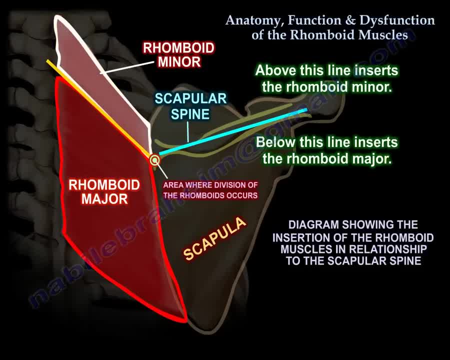 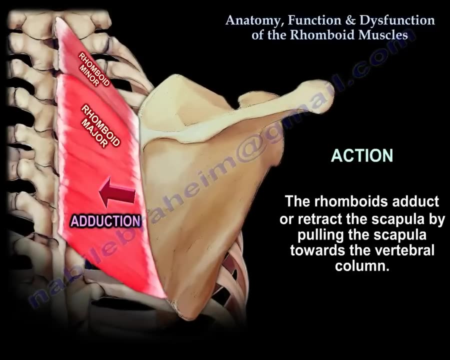 between the two muscles. Above this line inserts the rhomboid minor and below this line inserts the rhomboid major. Action Rhomboids adduct or insertion of the spine of the scapula. The rhomboids adduct or retract the scapula by pulling the scapula towards the vertebral. 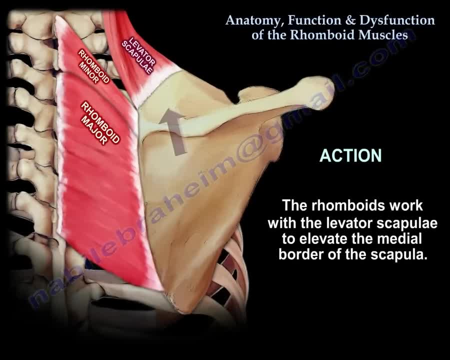 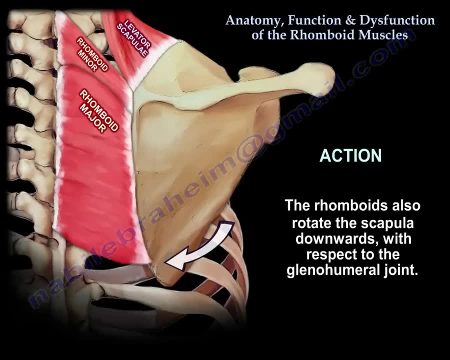 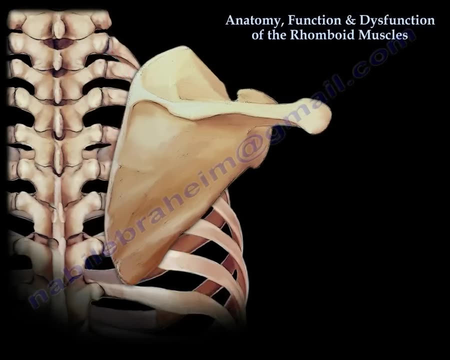 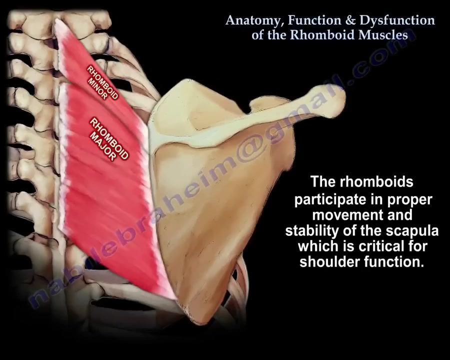 column. It works with the levator scapula to elevate the medial border of the scapula. It also rotates the scapula downwards with respect to the glenohumeral joint. The rhomboids participate in proper movement and stability of the scapula, which is critical. 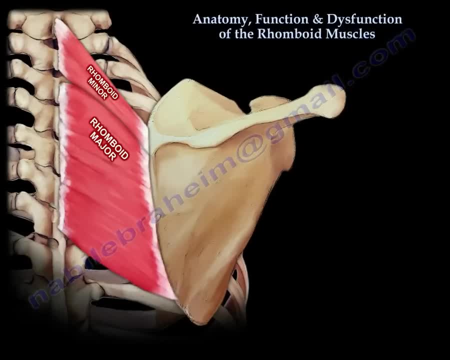 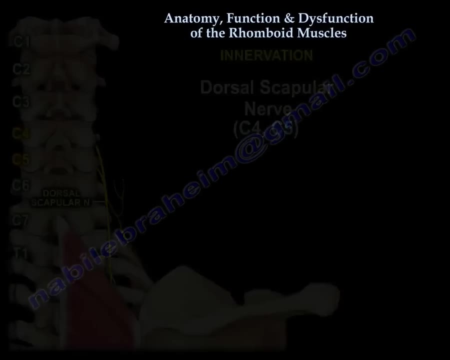 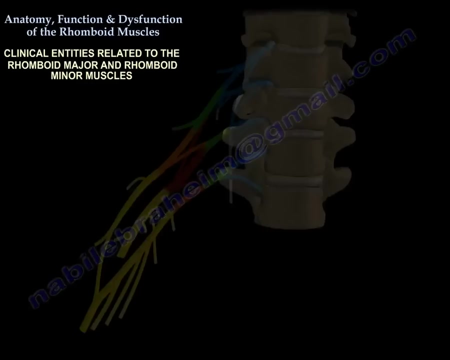 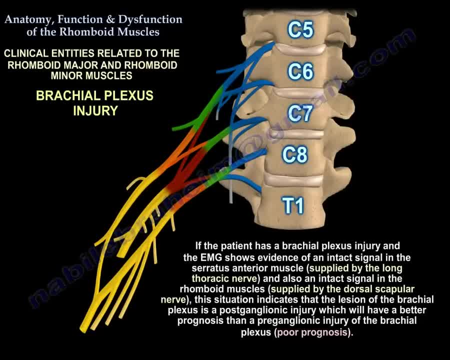 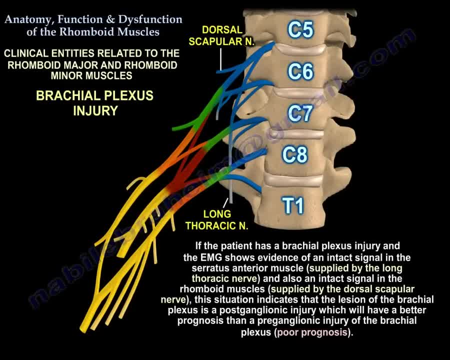 by the long thoracic nerve and also an intact signal in the rhomboid muscles which is supplied by the dorsal scapular nerve. This situation indicates that the lesion of the brachial plexus is postganglionic injury, which will have a better prognosis than the brachial plexus injury. 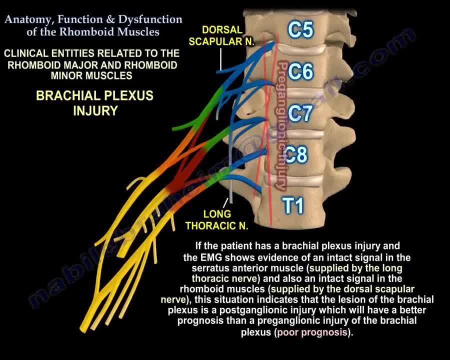 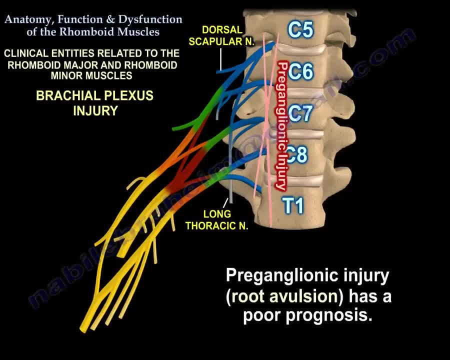 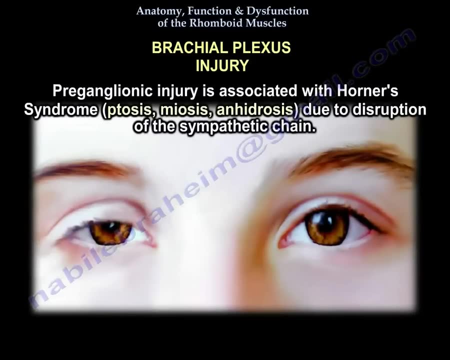 than the preganglionic injury of the brachial plexus. Definitely, the preganglionic injury will have a poor prognosis. The preganglionic injury is associated with Horner's syndrome, ptosis, meiosis and hydrosis. 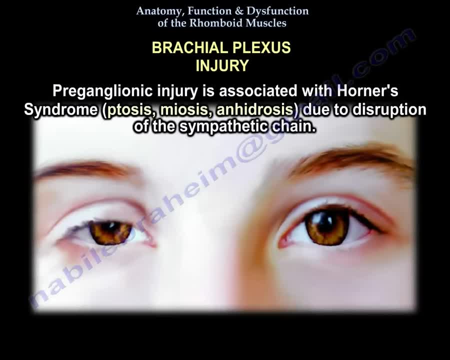 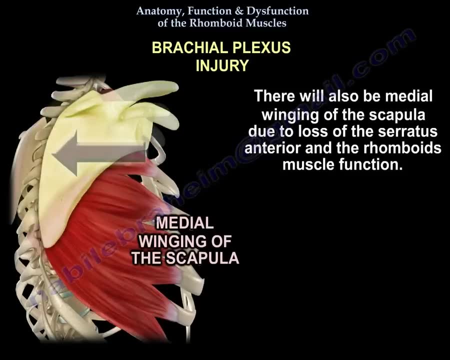 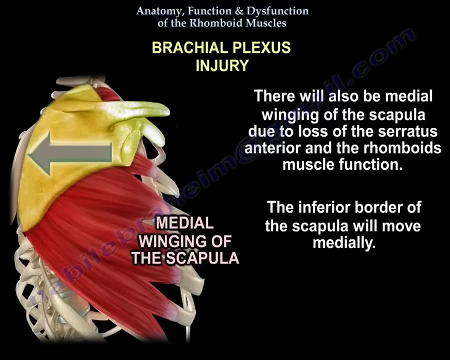 due to disruption of the sympathetic chain. There will be also medial winging of the scapula due to loss of the serratus anterior and the rhomboid muscle function. The inferior border of the scapula will move medially In the preganglionic injury of the brachial plexus. 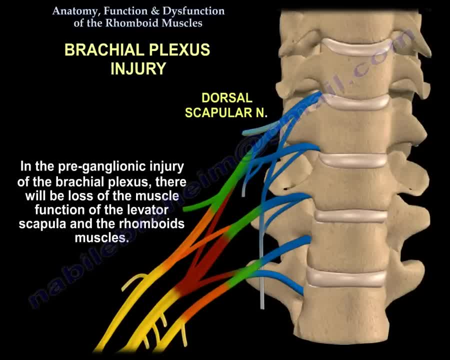 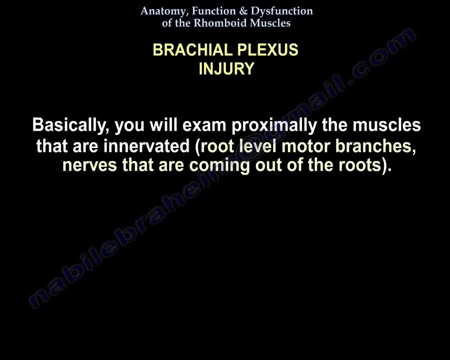 there will be loss of the muscle function of the levator scapula and rhomboid muscles. Basically, we will experience a loss of the muscle function of the levator scapula and rhomboid muscles. Examine proximally the muscles that are innervated. 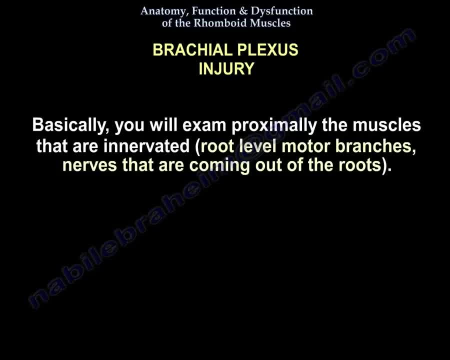 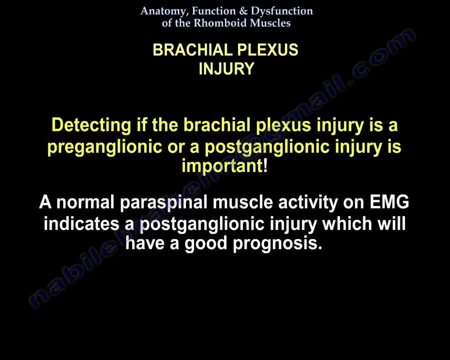 root-level motor branches, the nerves that are coming out of the roots. Detecting if the brachial plexus injury is preganglionic or postganglionic injury is important. A normal paraspinal muscle activity on AMG indicates a postganglionic injury. 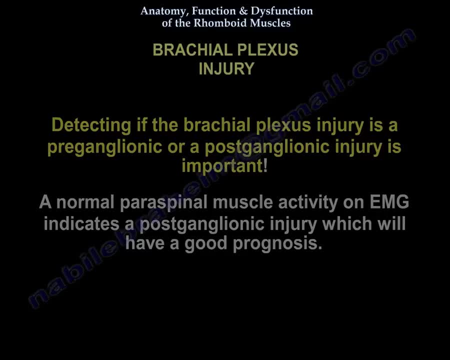 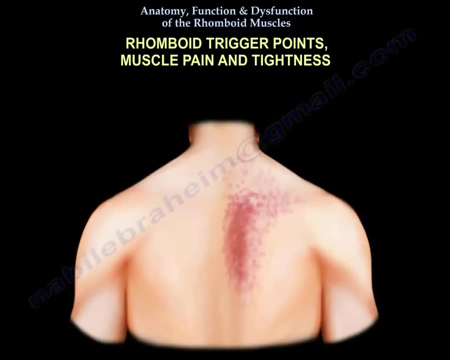 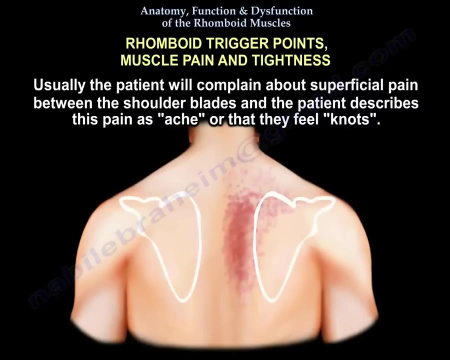 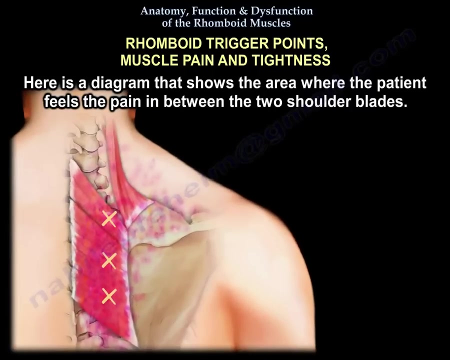 which will have a good prognosis. Another entity that is popular is rhomboid trigger points: muscle pain and tightness. Usually the patient complains about superficial pain between the shoulder blades. Patients describe it as an ache, or they feel knots. Here is a diagram that shows the area where the patient feels the pain in between the shoulder blades. 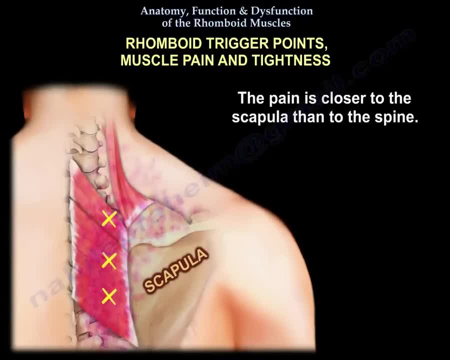 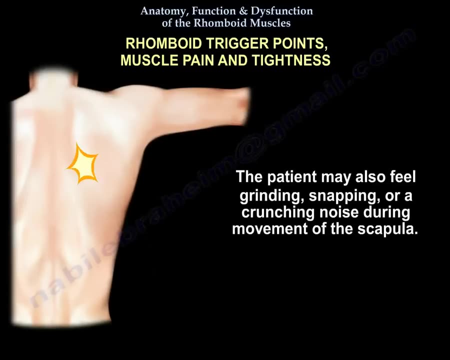 The pain is closer to the scapula than to the spine. The pain occurs especially at rest, and movement does not influence the pain. The patient also may feel grinding or snapping or a crunching noise during movement of the scapula, And in this case you need to rule out a scapulothoracic impairment. 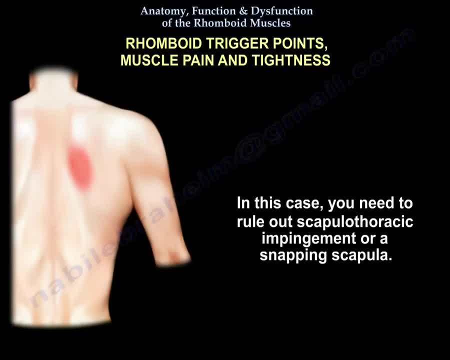 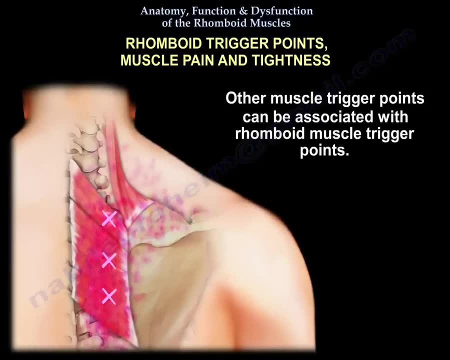 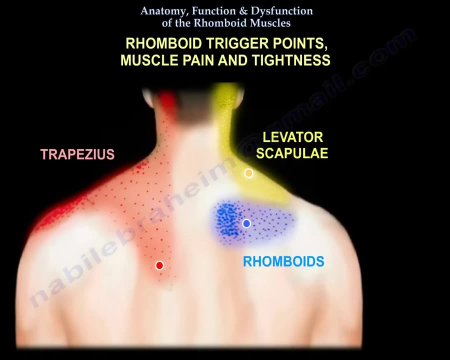 And in this case you need to rule out a scapulothoracic impairment or a snabbing scapula. Other muscle trigger points can be associated with rhomboid trigger points, such as pectoralis, major levator scapula and trabezius. 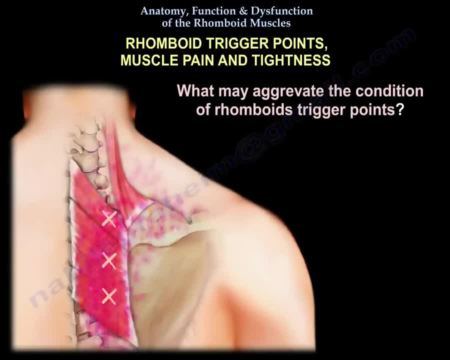 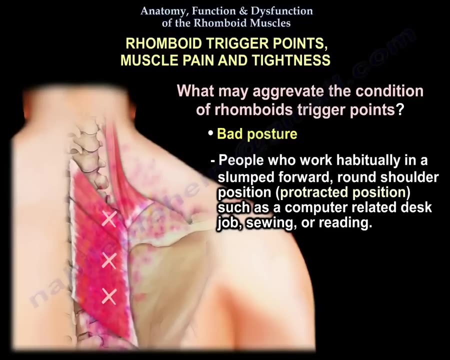 So what aggravates the condition of rhomboid trigger points? Painters that are holding their arm above the head for a long time- Bad posture, like the people that work habitually in a slumped forward round shoulder position, which is a protracted position, such as in people that work on a computer or a desk job. 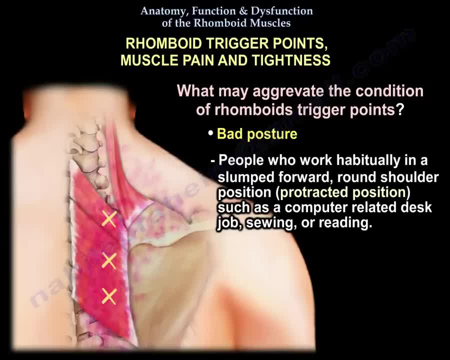 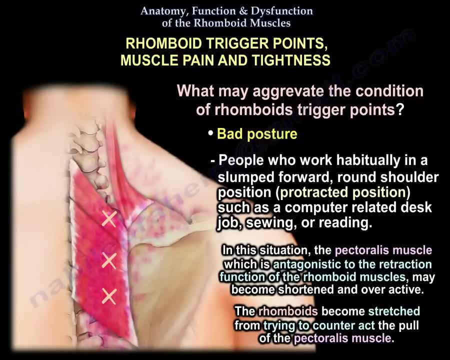 or people that are sewing or reading. In this situation, the pectoralis, which is antagonistic to the retraction function of the rhomboids, can be a trigger point for this muscle to become shorted and overactive And the rhomboids become stretched trying to counteract the pull of the pectoralis. 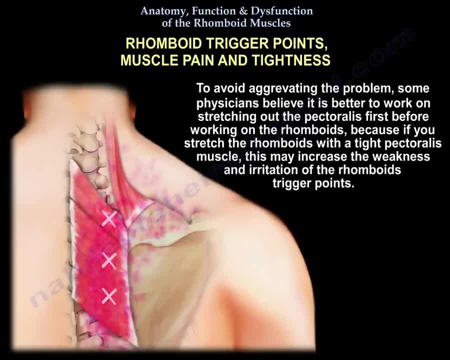 How to avoid aggravating the problem. To avoid aggravating the problem, some people believe it is better to work on the pectoralis first before you work on the rhomboids, Because if you stretch the rhomboids with tight pectoralis muscle, this may increase the weakness. 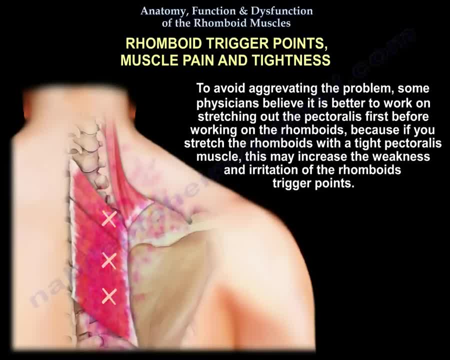 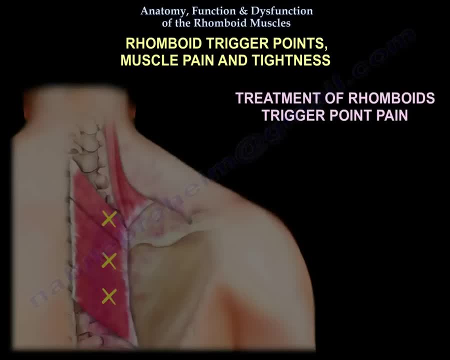 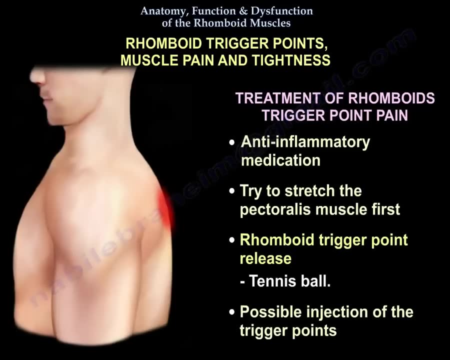 and the irritation of the trigger points. So how do you treat rhomboid trigger points? You give the patient anti-inflammatory medication. You may try to stretch the pectoralis first. You may do rhomboid trigger point release. You may treat it by a tennis ball.